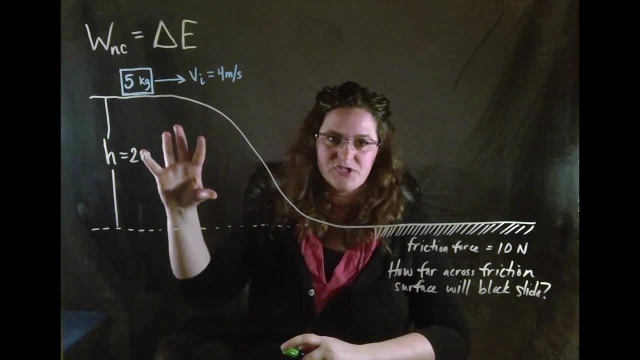 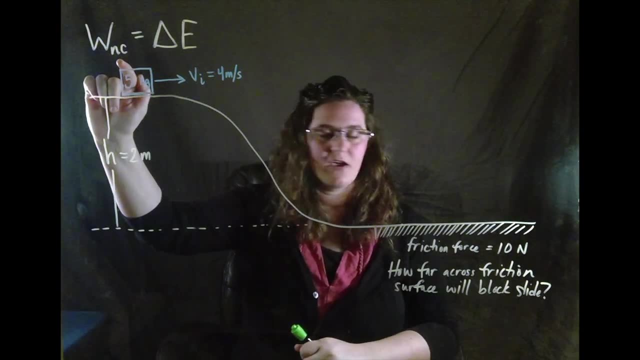 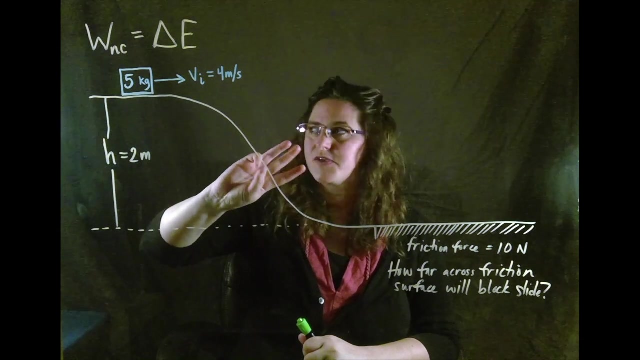 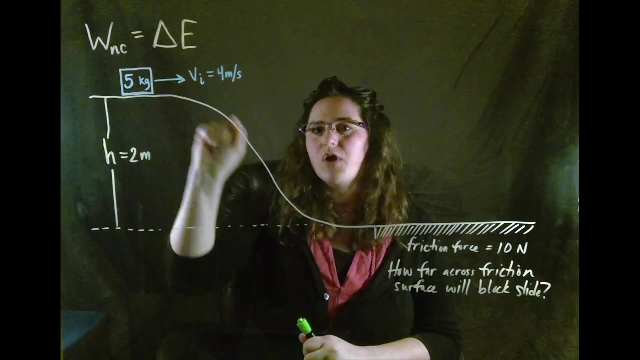 to find. Let me show you how to use the equation that is necessary here. This equation says that the work done by the non-conservative forces are responsible for the change in mechanical energy. So first we have to find three different things. We have to figure out what work is done by the non-conservative forces in this system. 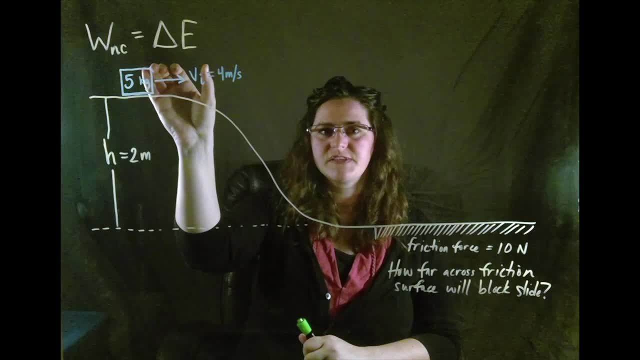 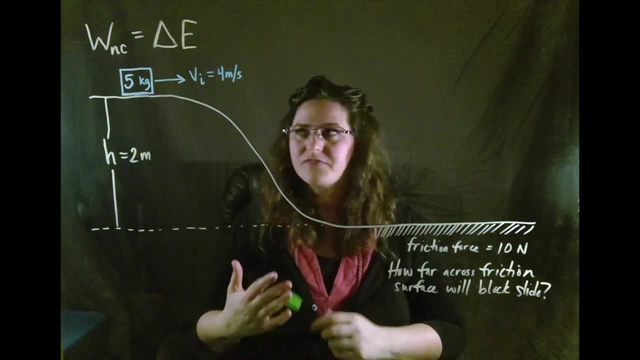 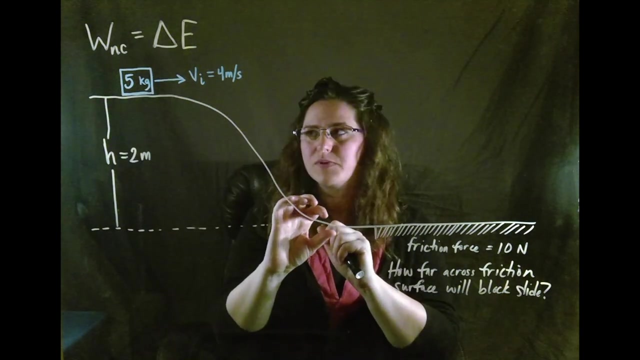 We also have to figure out what the final energy content of the system is, That's, mechanical energy, And what the initial energy content is. So let's draw the final position of our block here. Our block slides down the slope. And the really cool thing about these problems: 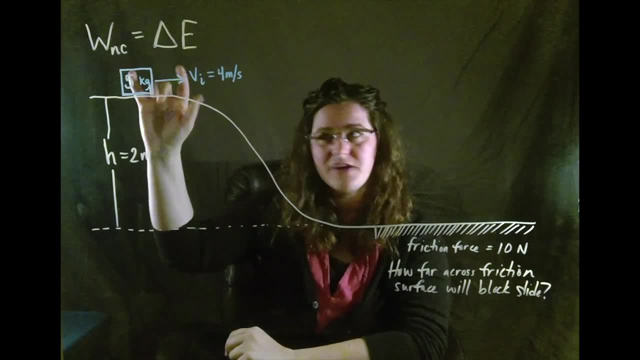 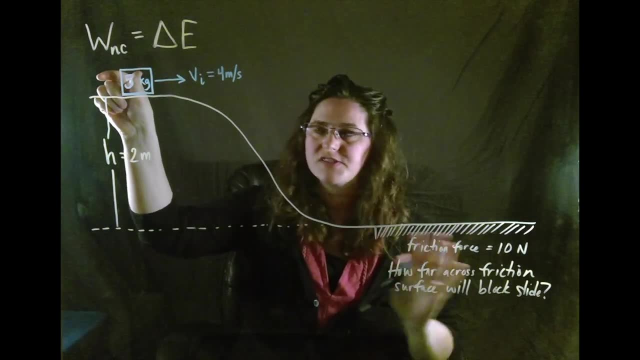 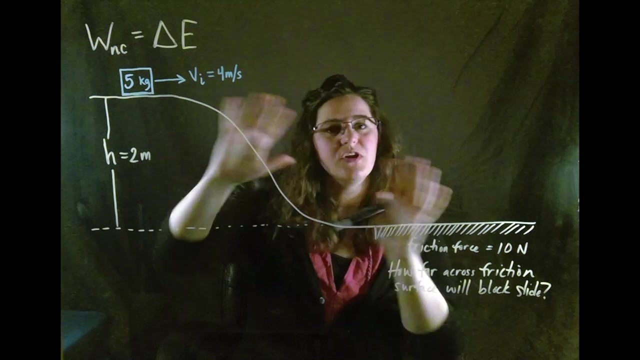 is, you don't have to care about anything else besides the three elements that I just told you about Work done by the non-conservative forces- and the only non-conservative force here is friction And the final energy minus the initial energy, And we don't care what happens to the block. 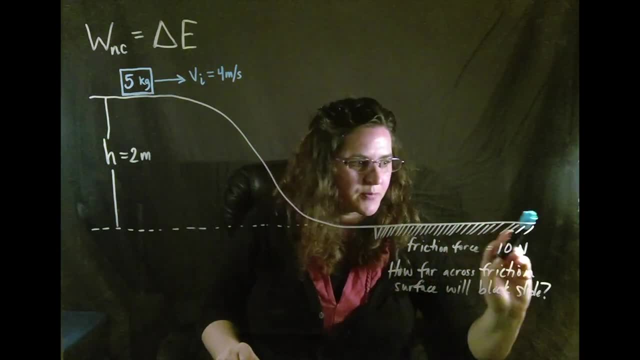 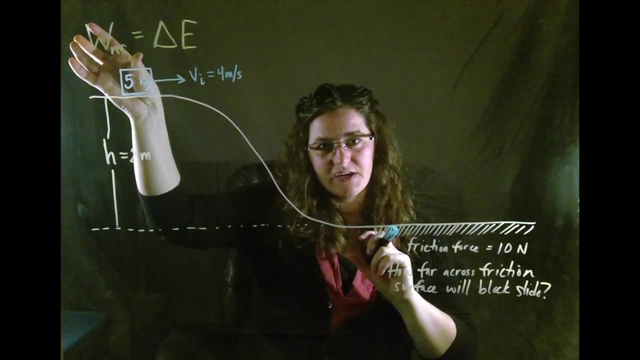 in between. It could go around a loop-de-loop and end up right down here, and it wouldn't matter. What only matters is the initial energy, the final energy and the work done by the non-conservative forces, In other words, the energy taken from the system. That's what's. 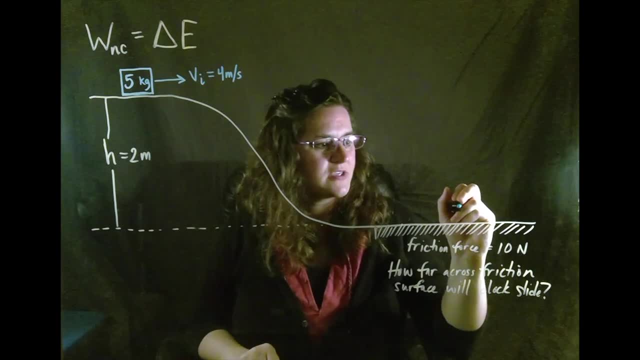 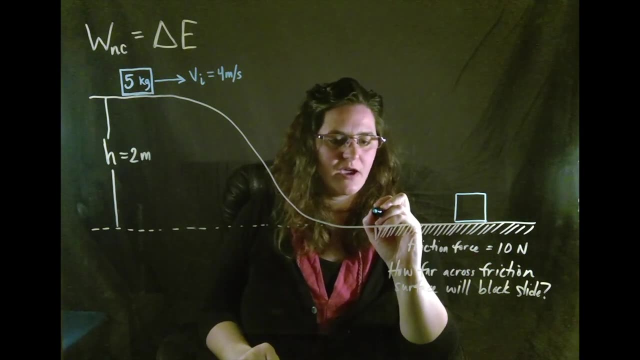 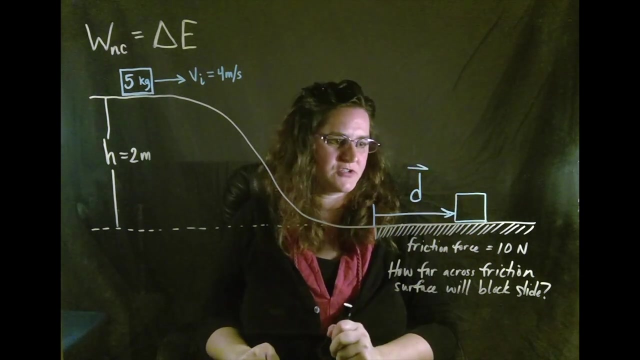 responsible for the change in energy. Okay, so the block ends up. let's just draw the block here, Let's say that the block ends up right there, And so we're being asked to find this distance, this displacement. We're going to call that a vector d. 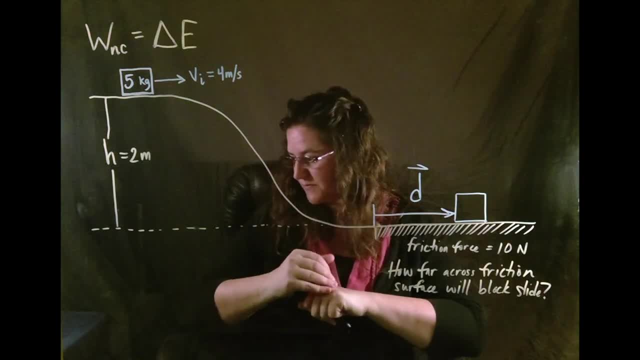 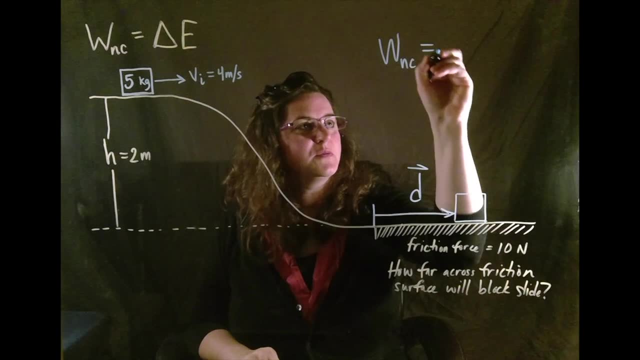 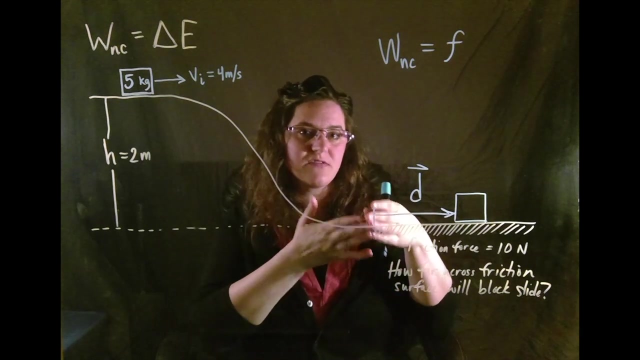 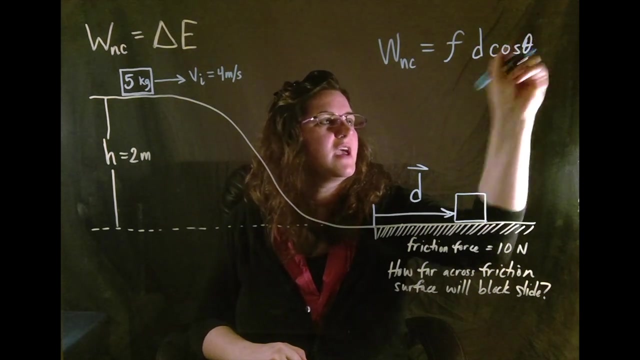 Now let's go ahead and find the work done by the non-conservative force. So we know that work, the work done here, is equal to The force. So it's equal to a force times, a displacement times, the cosine of the angle between them. Okay, so the work times, the displacement times, the cosine of the angle. 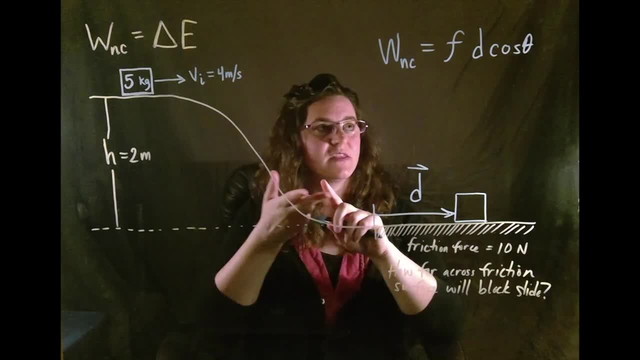 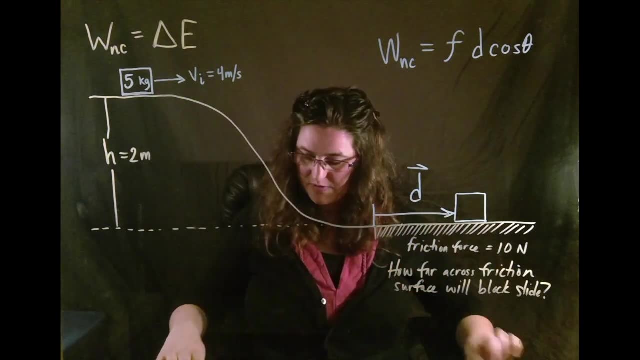 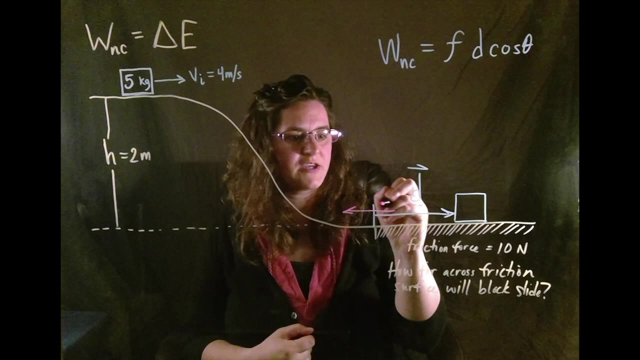 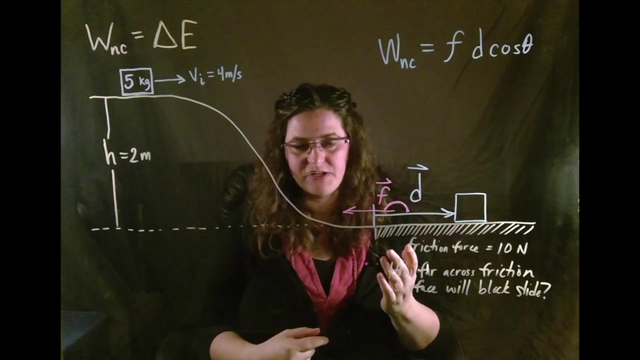 between the work, I'm sorry, between the force and the displacement. Okay, so our displacement was pointed this way And our force is pointed the opposite direction from the motion because it's friction, So our friction force is actually Okay In that direction. Now you can see that the angle between these two forces is 180 degrees. 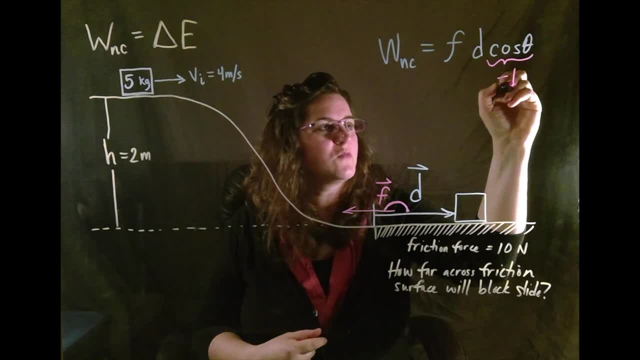 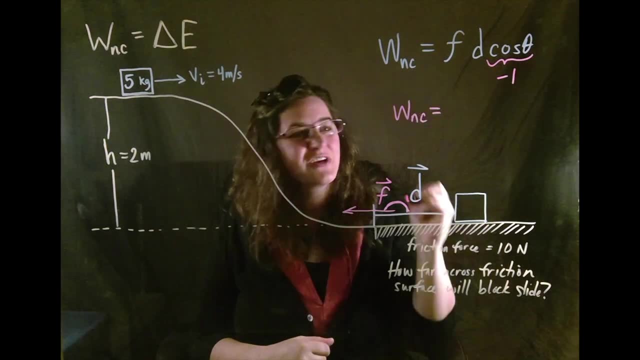 or pi. So what we're going to get from this is negative one. So really, the work done by the force. it makes sense that the work done by the non-conservative force is something that takes energy from the system, So we're going to have negative, the friction force. 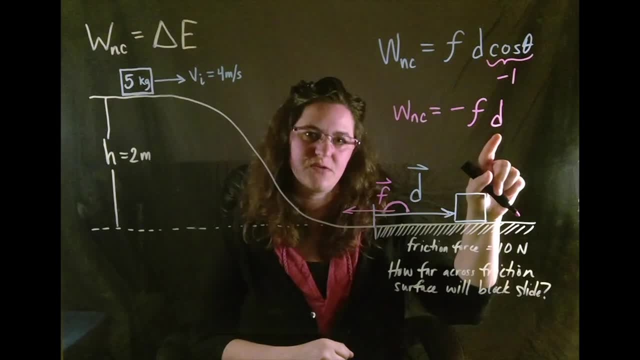 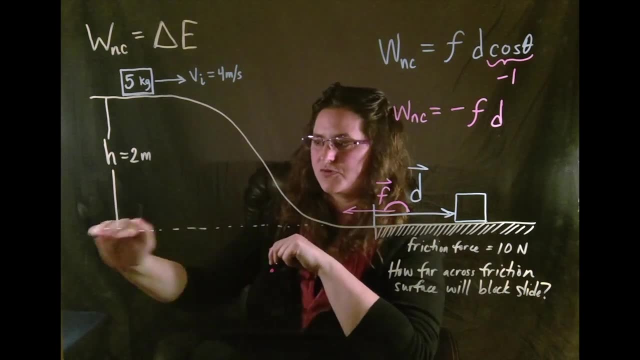 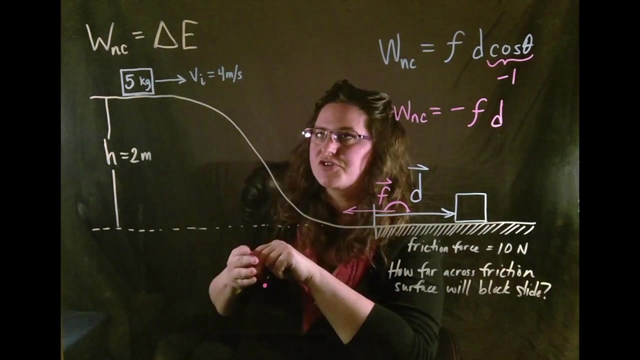 which we're given. it's 10 Newtons times d, which is the thing that we're trying to solve for The initial system has a potential energy because let's put our zero potentional gravitational potential energy here, and so we are up by two meters. So our initial energy in this 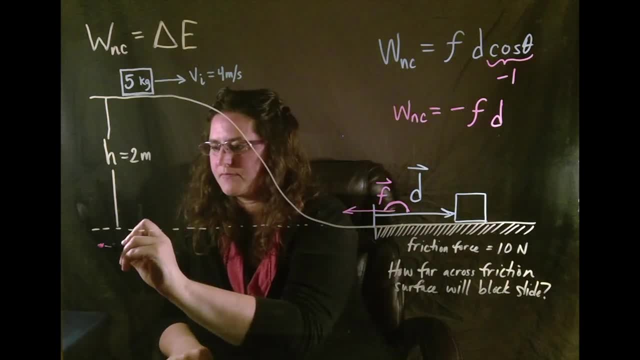 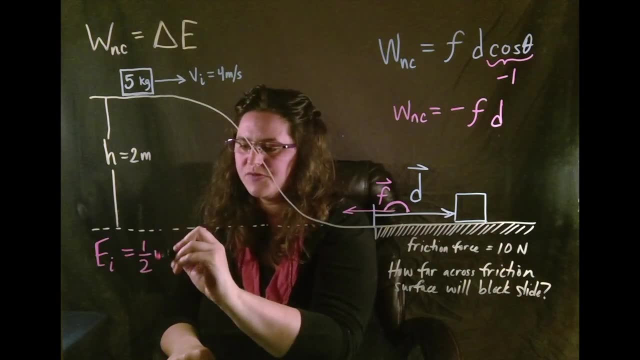 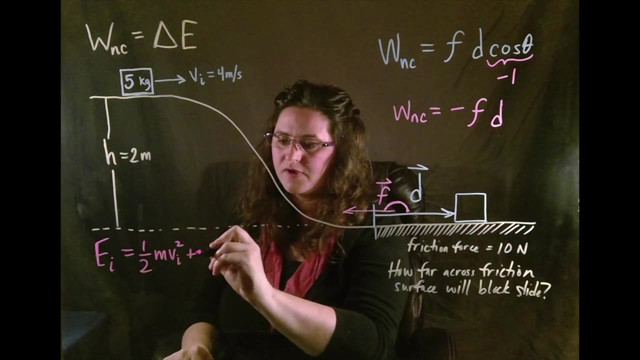 system is. let's see: E initial is equal to. It's got kinetic energy. one half M V initial squared Okay Okay. so it's got some potential energy. this is a positive 9.8, because it's just an. 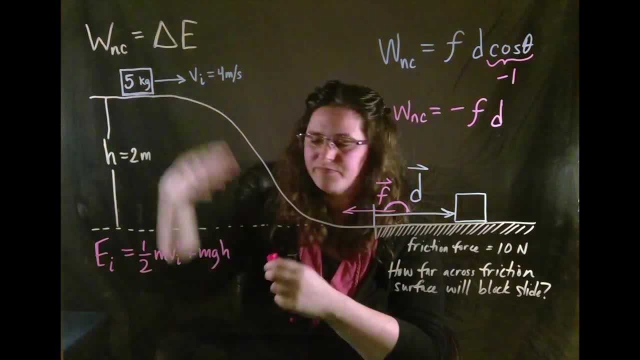 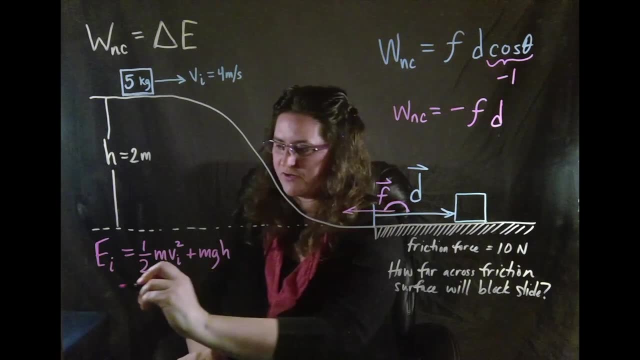 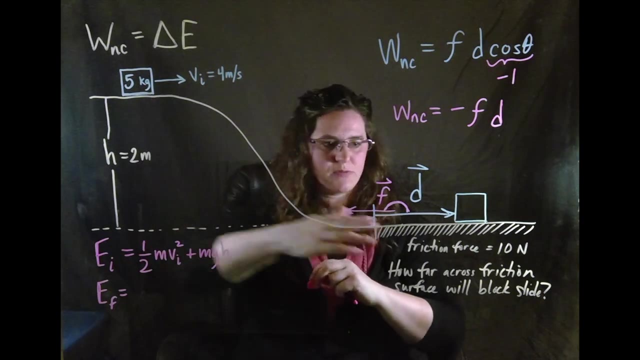 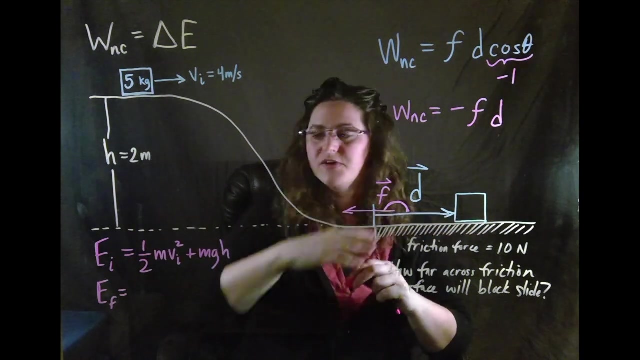 amount that is up. so this is our initial energy. this is a positive number. the final energy, the final energy is equal to well. it has stopped moving and it has come to where we called our zero potential here. so it has no potential, it has no kinetic there. 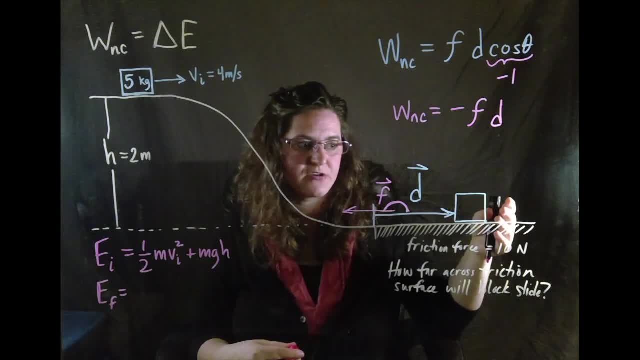 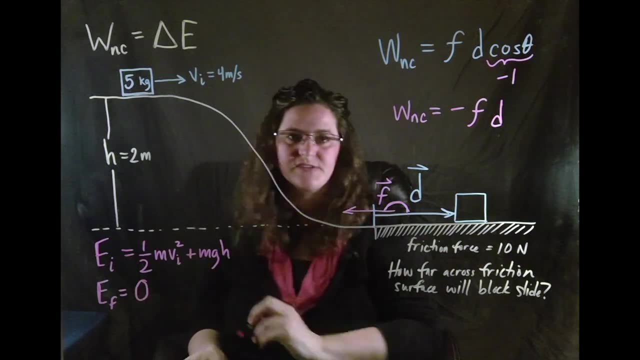 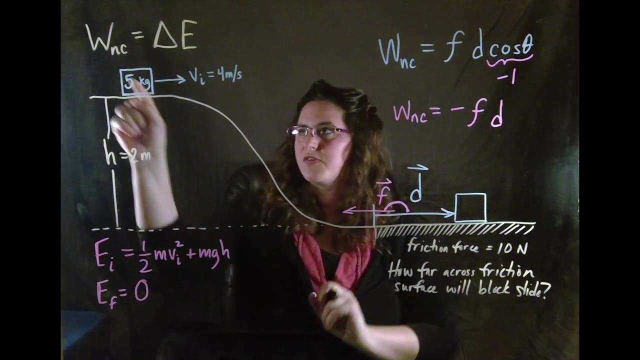 were no springs in this system, and it's not compressing a spring here, so there's no potential energy from the spring either. those are the only forms of energy that we can have, so the final energy is zero. all right, so let's put everything together. we were told that the work done by the non-conservative 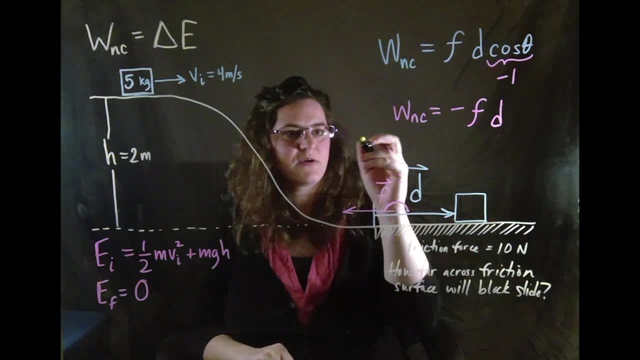 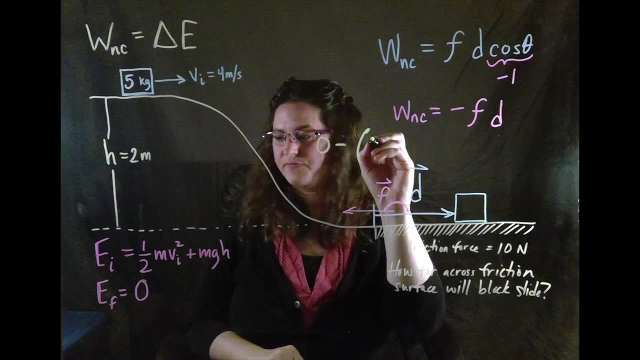 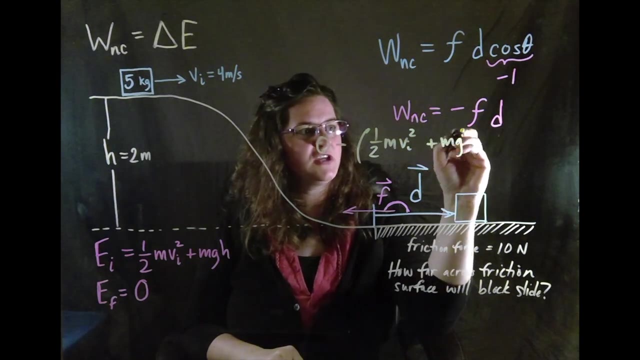 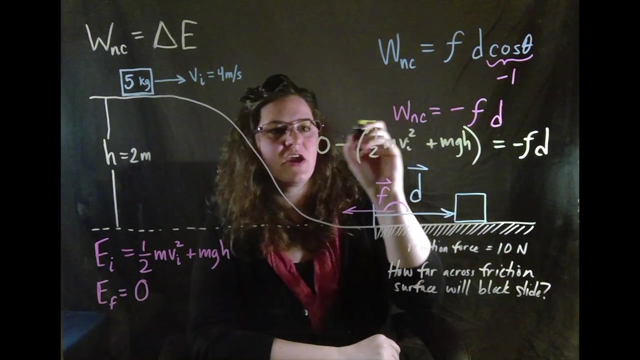 force is equal to the change in energy. all right, so zero minus. I'm rewriting this equation here. the initial energy: 1, half and bi squared plus mgh, this is equal to negative F, D, and now we have an equation that we can solve for D here.